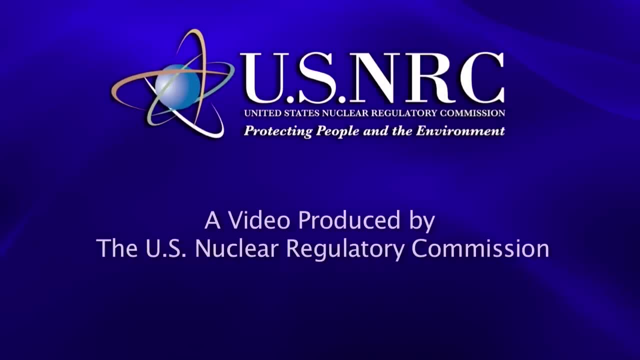 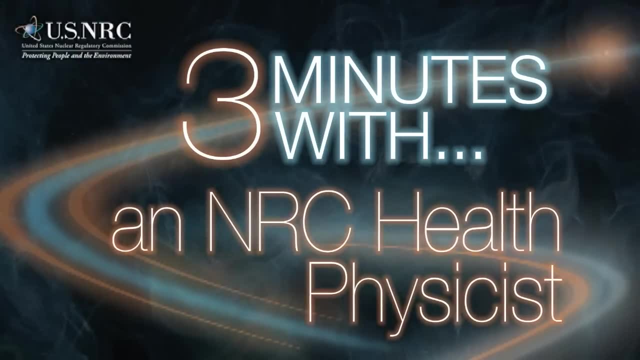 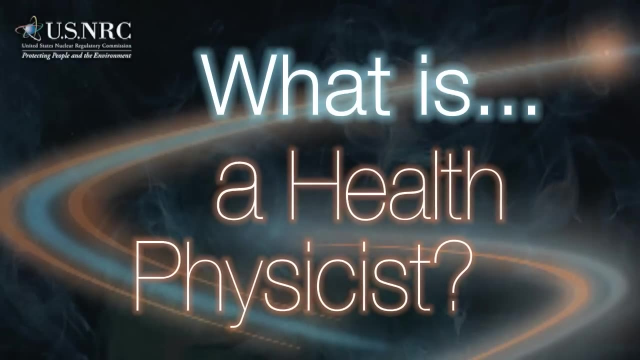 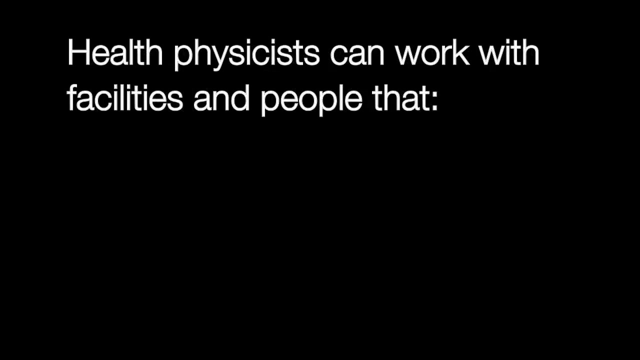 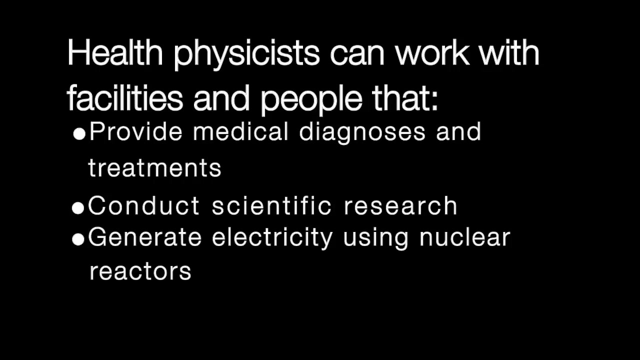 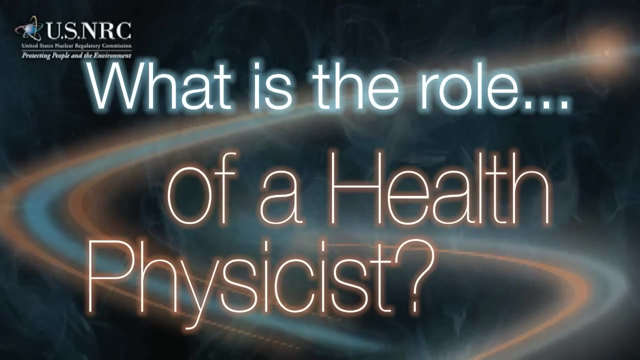 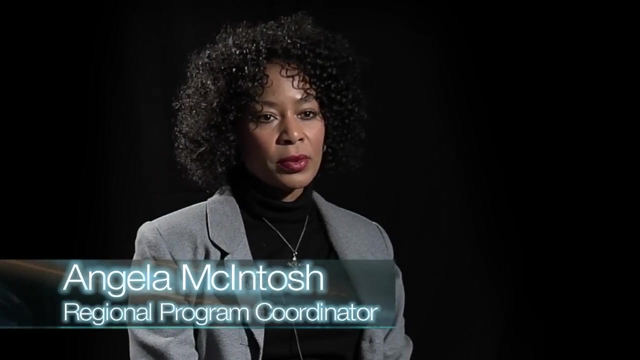 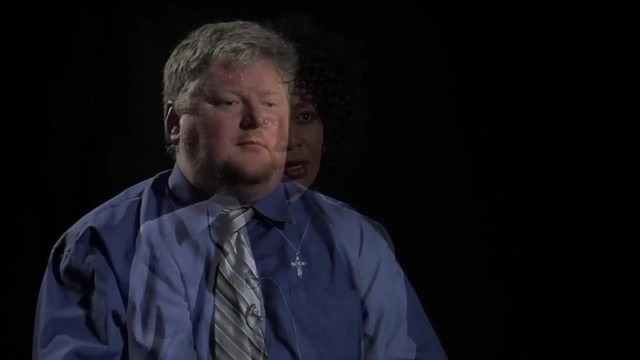 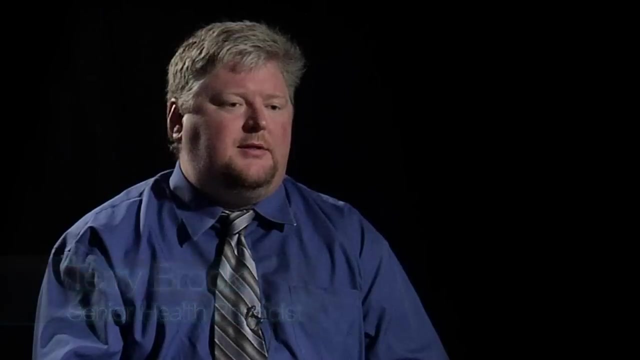 Thank you for watching. The role that HP professionals play in society is that they help ensure that wherever radioactive material is used, it is used safely and responsibly. The role of the radiation protection professional in our society is an important one, because what it does is it allows for the use of these materials. 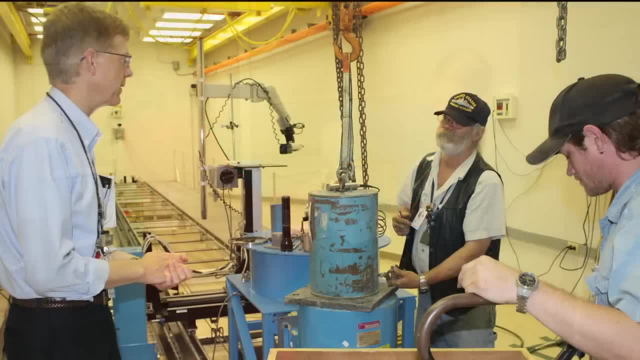 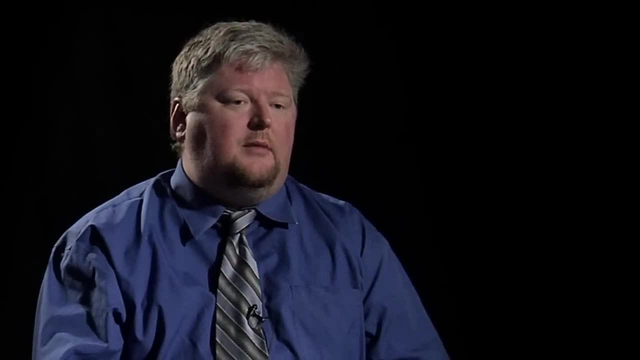 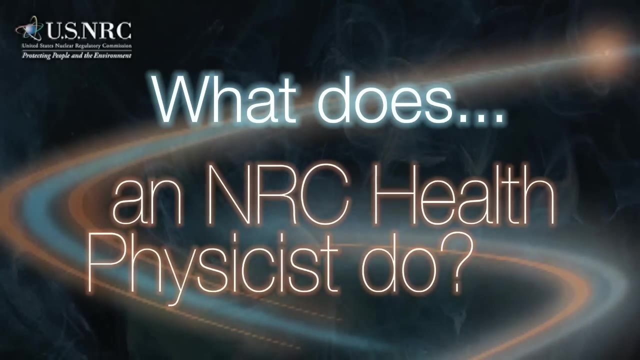 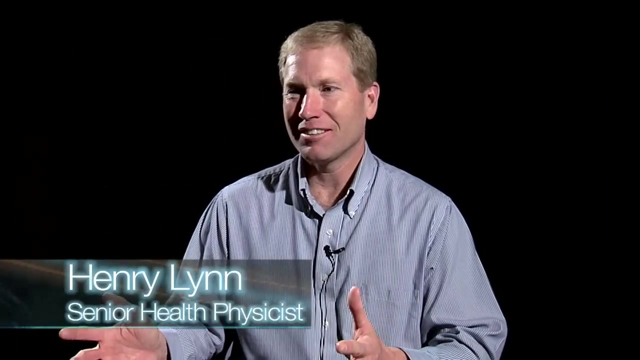 Beneficial technologies, either through medicine or research, or industrial uses or energy production. it allows for those uses while protecting against the potential harmful effects of radiation exposure. Well, I like to think that nuclear regulation wouldn't be necessary if not for radiation. So radiation protection really is the backbone. 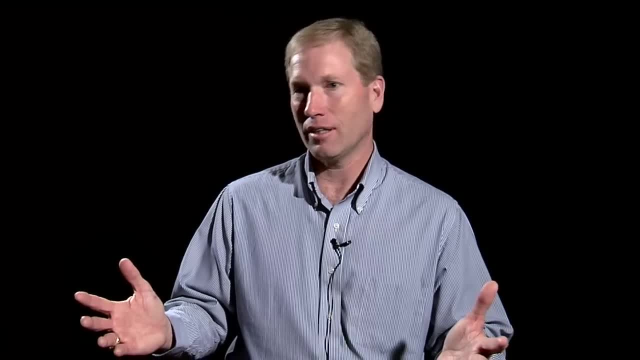 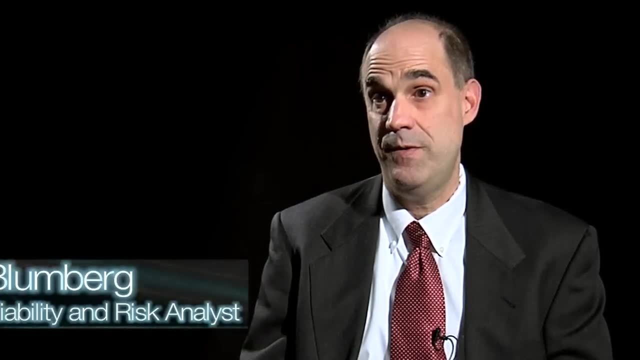 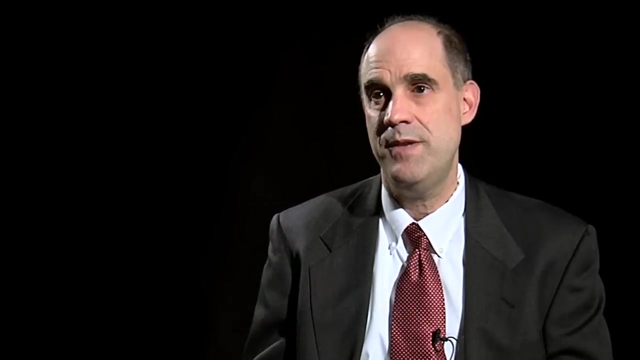 To our agency. all of the regulations in the end are about controlling radiation and the radioactive material associated with it. My main responsibilities for day-to-day are basically in the area of licensing. We receive license amendments from nuclear power licensees that want to make changes to their facilities. 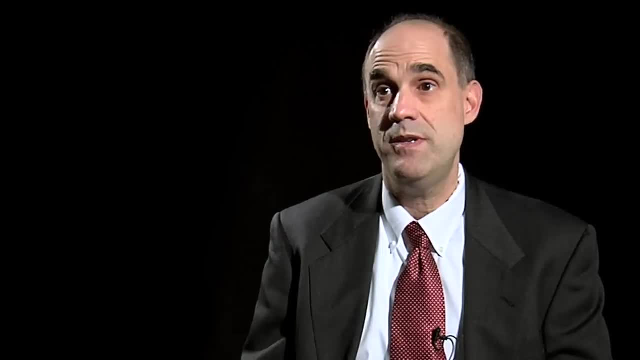 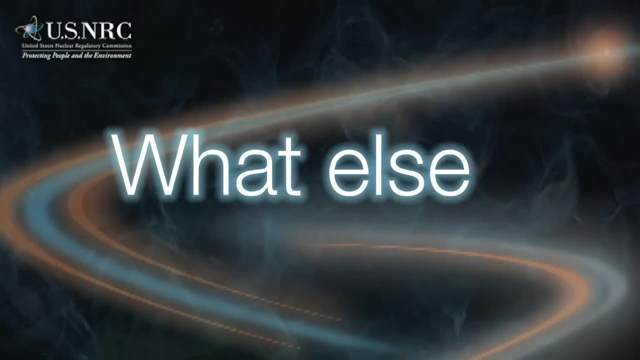 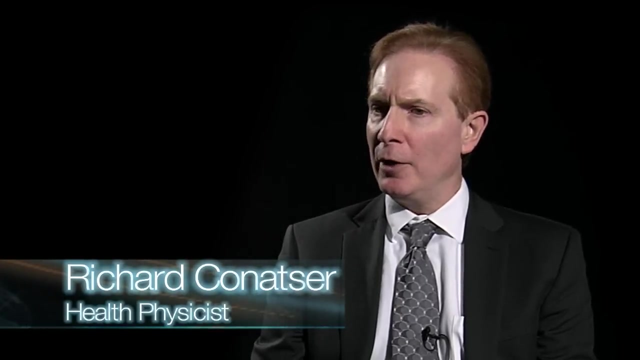 And we receive those license amendment requests And my job is to review those against the regulations And we have to make sure that they continue to meet those regulations. Since I'm at headquarters, generally the regions have their own expertise out there- They can generally do all these inspections on their own. 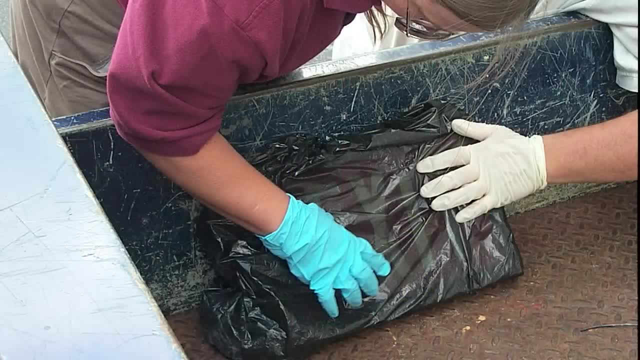 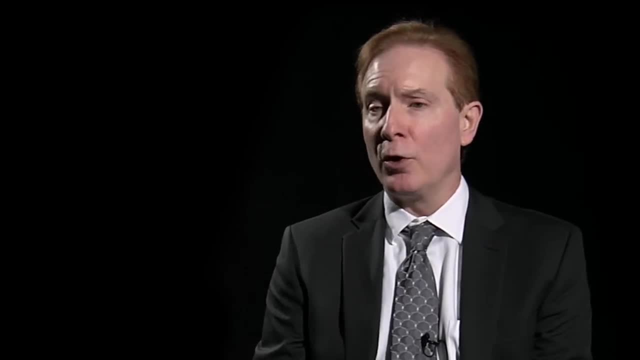 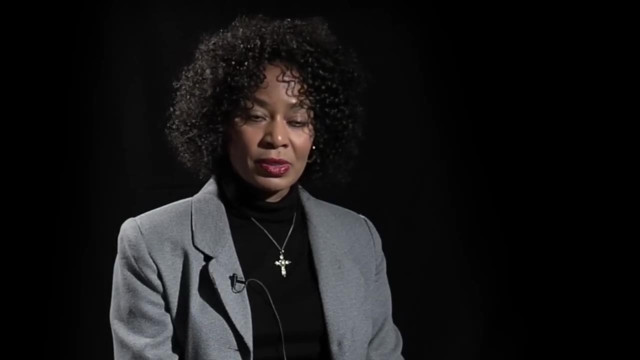 They generally will call me and say: well, we have an inspection where there will be probably lots of questions or we want any particular expertise in an area that you are well versed in. Sometimes we do have conversations, controversial issues that we face, particularly in the medical arena, that call for us to